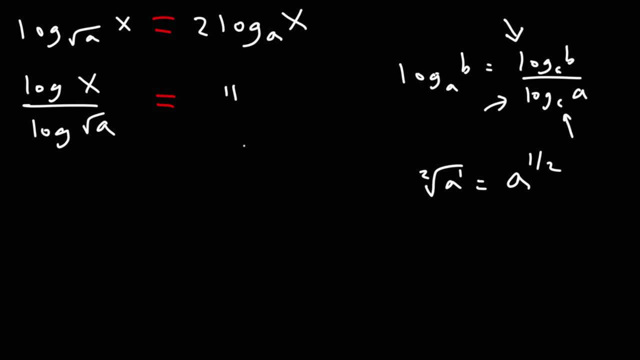 the radical, it's assumed to be a 2. So it's A to the one-half. So we can rewrite this as log X over log B. So we can rewrite this as log X over log B. So we can replace A to the one-half. Now log A raised to the X, This is equal to X log A, That's. 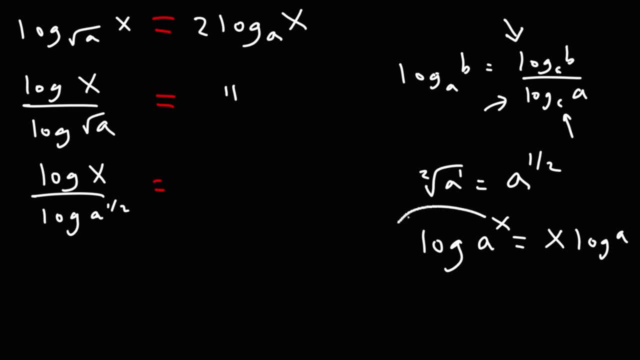 another property of logs. You can move the variable to the front, And that's what I'm going to do here. I'm going to take the one-half exponent and move it to the front. So now I have log X over one-half log A. 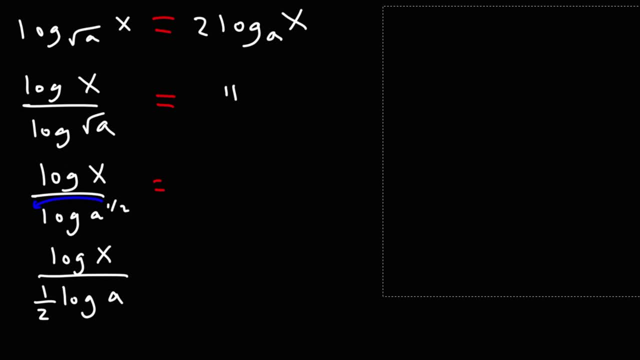 Now to get rid of the one-half and the bottom, we're going to multiply the top and the bottom by 2.. 2 over 2 is 1.. So if you multiply anything by 1, you don't change the value of that thing. 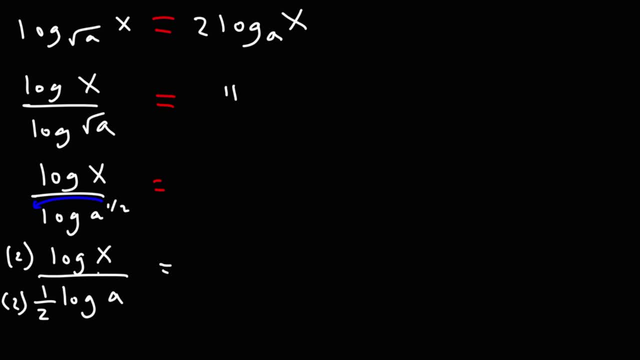 you're multiplying by. So by multiplying this fraction by 2 over 2, we are not changing the value of the fraction. Now, 2 times the half is 1.. So we're going to get 2 times the log X over log A, And I'm going to write this as 2 times log X over log A. Now I'm 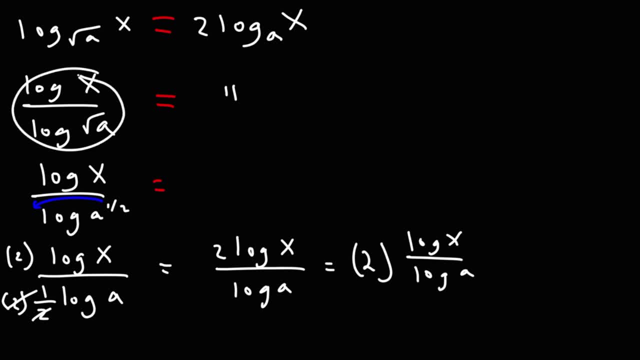 going to use the change of base formula to go back from a division of 2 logs into a single log. So the one that goes on top goes here. The bottom becomes the base And then I'm going: So this is going to be 2 times log. this is on the bottom, so a is going to be the base. 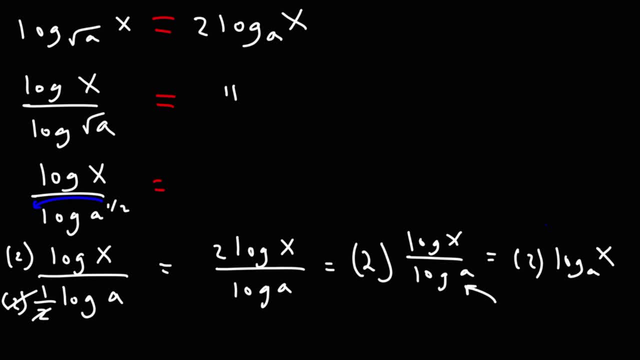 and then x, which is equivalent to the expression on the right side. So that's how we can prove that this particular logarithmic equation is indeed true. Now let's work on another example. Let's say we have log base a raised to the 9th power of x, cubed. 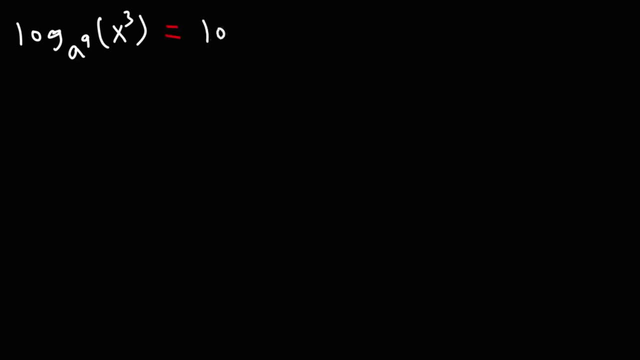 and we're going to set that equal to log base a of the cube root of x. Feel free to pause the video and work on this example problem. Go ahead and prove whether or not, if this mathematical system is true, this statement is true. 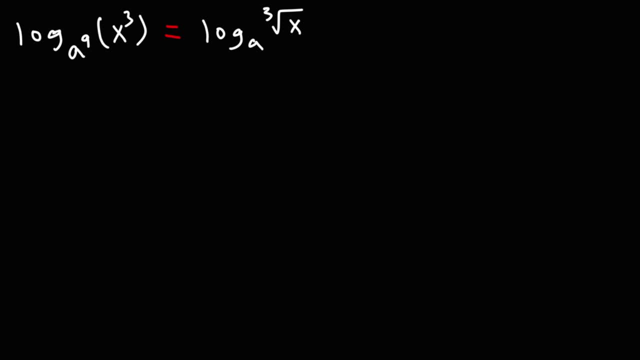 By the way, for those of you who are studying logarithmic equations or just logs in general, and if you have a test coming up, I'm going to post a lot of links in the description section below this video that has to do with logarithms. 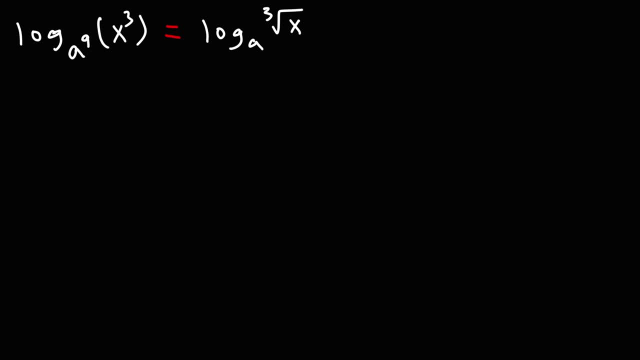 So for those of you who need help with other topics involving logs, feel free to check out the description section below. So for this problem, we're going to use a simple formula. So for this problem, I'm going to start from the left side. 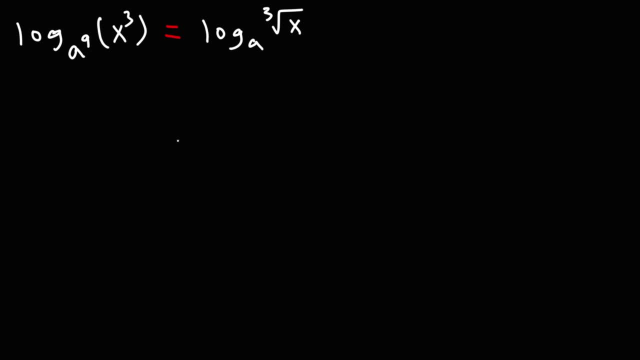 I'm going to convert it to the right side. So, just like before, let's use the change of base formula. So this is going to be log x cubed, divided by log a to the 9th power. You know, once you do one example, the other examples, they become easier. 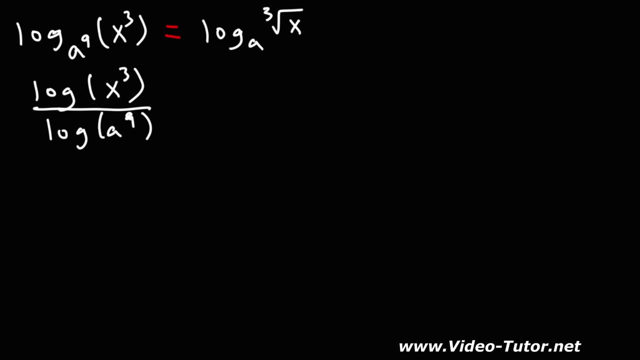 because now you know the pattern that you need to follow. Now, just like before, we're going to convert it to the right side, So we're going to move the exponents to the position in front of the logs. So log x cubed becomes 3 log x and log a to the 9th becomes 9 log a. 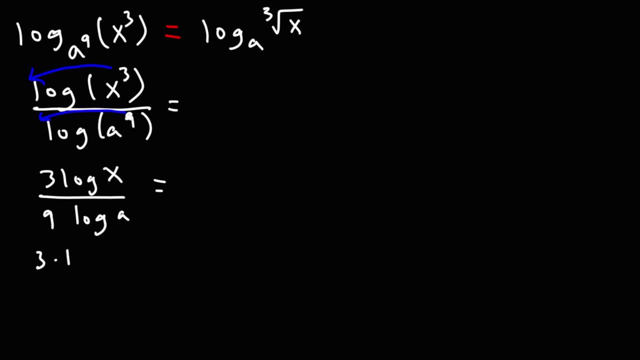 Now 3, I'm going to write that as 3 times 1, or, better yet, 1 times 3.. 9, I'm going to write that as 3 times 3.. So I'm going to cross out a 3, and notice that I'm left with 1, 3rd in front. 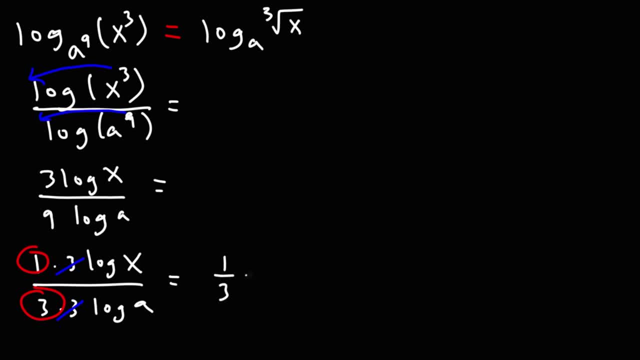 And I'm going to move that in a separate fraction. So this is going to be 1, 3rd times, log x over log a. Now what I want to do, because I have a division of two logs, but my final answer only has a singularity. 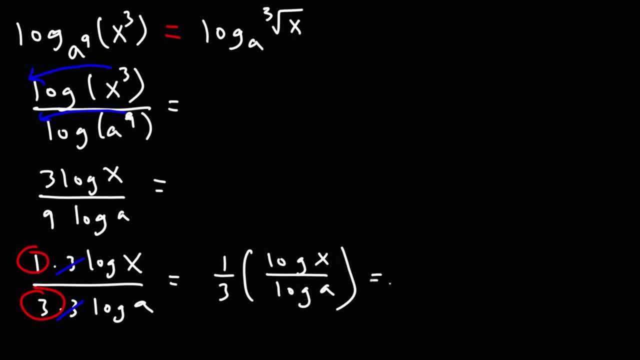 I need to use the change of base formula to go back to a single log. So this is going to be 1. 3rd log, base a of x. Now this exponent, I mean this coefficient rather or constant. I'm going to move it to the exponent position. 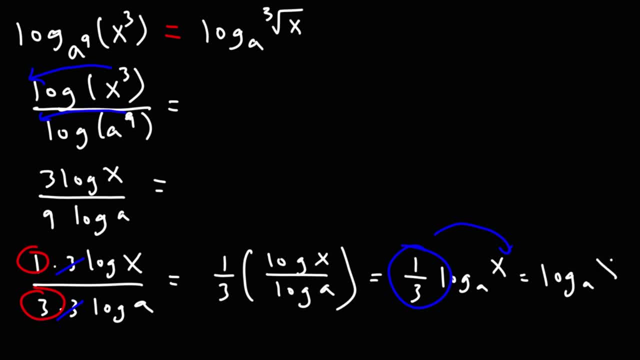 So this becomes log base a of x to the 1: 3rd. Now x to the 1: 3rd is the cube root of x. So we can write our final answer like this: Log base a, cube root of x. 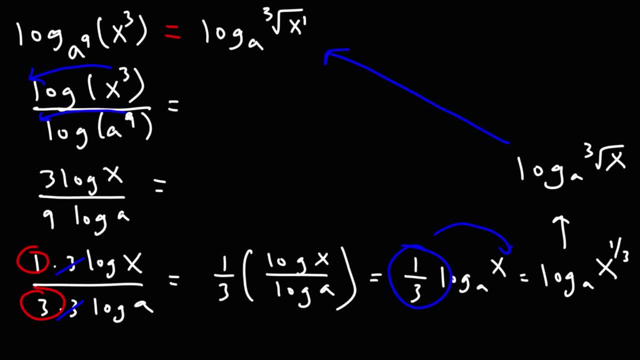 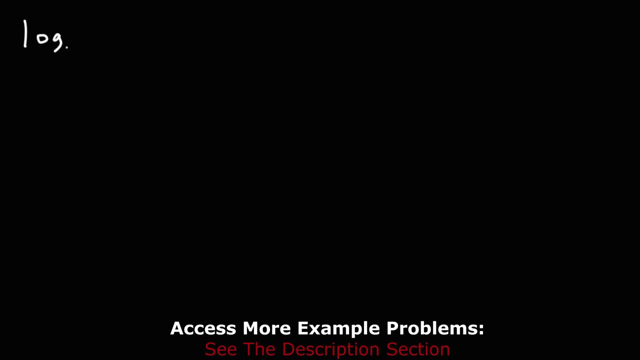 And, as you can see, the two. this equation is a true equation, It's correct, It's been proven true. Now let's move on to our last idea, To our last example for this video. Feel free to try this problem. 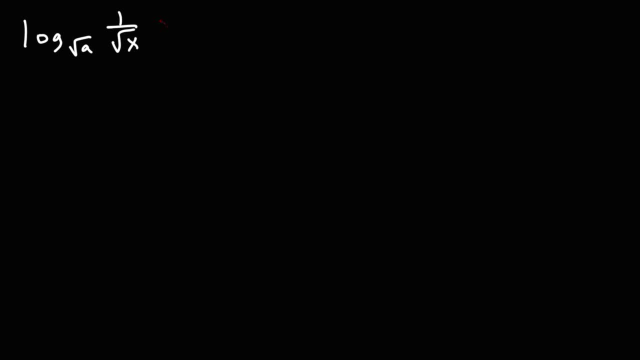 So we have log base square root of a of 1 over square root x And let's see if it equals negative log base a of x. Go ahead and try that. So let's begin by using the change of base formula. We'll take this single log and we'll write it as a division of two logs. 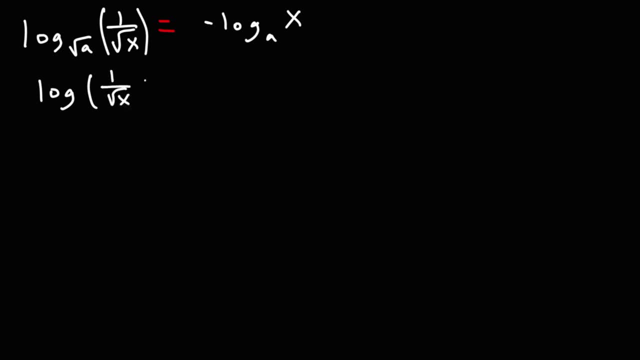 So this is equivalent to log 1 over the square root of x divided by log square root a. Now the square root of x is x to the 1 half And the square root of a is a to the 1 half. Now this x. I'm going to move to the top of the fraction. 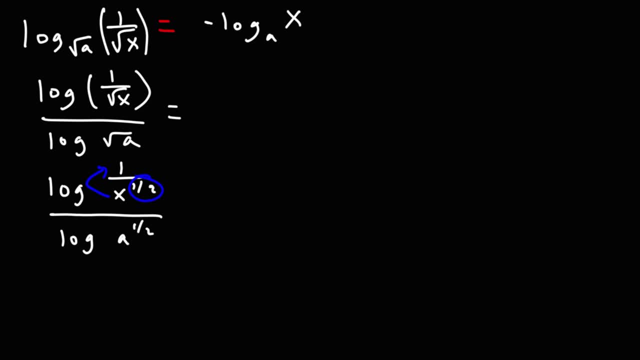 And when I do that, the exponent is going to change from a positive value to a negative value. So instead of being positive 1 half, it's now going to be negative 1 half. Next, we can move all of the exponents to the front of their respective. 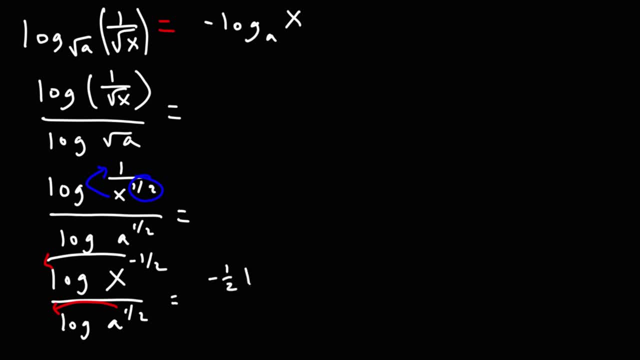 so we're going to have a negative 1 half times log x over positive 1 half times log a. Now 1 half divided by 1 half is 1, but we do have a negative sign in front of that. So right now we have negative log x over log a.